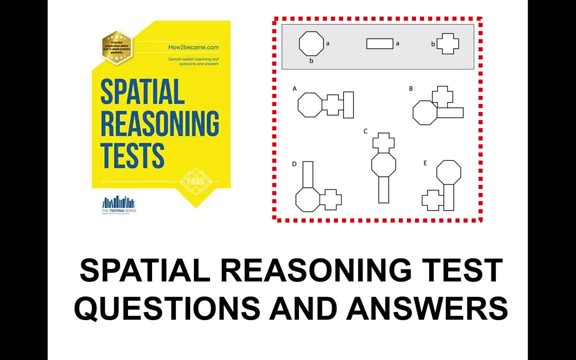 Hi everyone, My name is Richard McMunn from the career guidance company HowToBecomecom, and in this presentation I'm going to give you some sample spatial reasoning test questions and answers, explain how to get them correctly and give you a few tips along the way, Please. 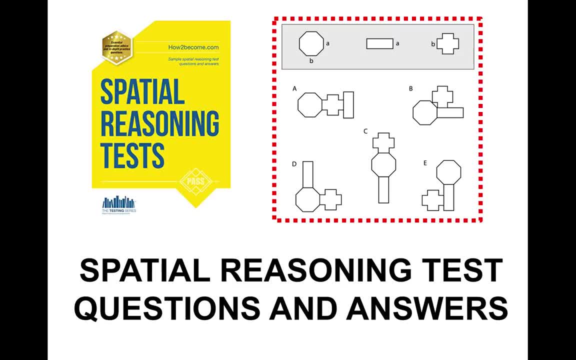 watch the video from beginning to end, because I'm also going to tell you where you can download some sample test questions to help you during your exam. OK, so spatial reasoning tests can be relatively difficult to answer because you have to use your mind, You have to, basically. 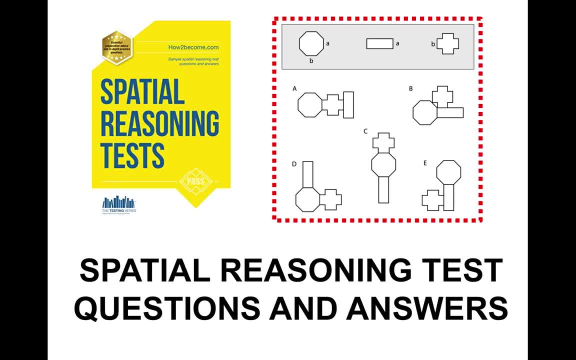 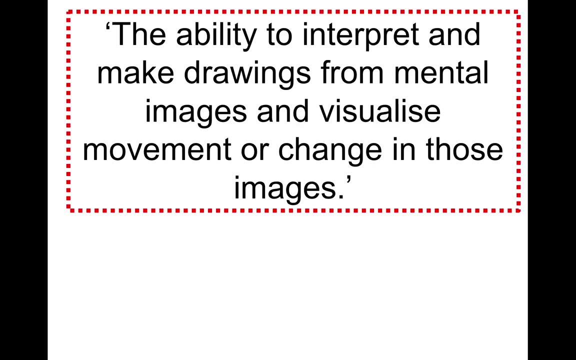 interpret shapes and visualize how a shape might rotate or when you put shapes together. So there's many different variations of spatial reasoning tests And basically, spatial reasoning is your ability to interpret and make drawings from mental images and visualize movement or change in those images. And the only way that you're going to improve your scores is 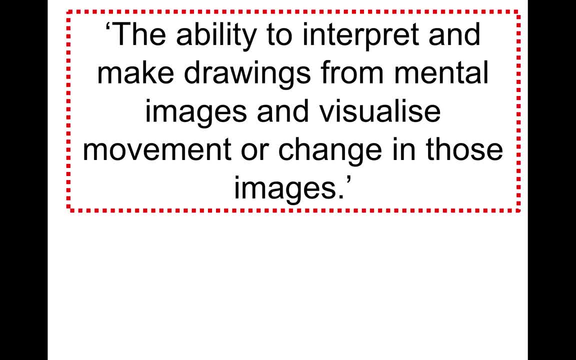 to do lots of practice. OK, There's no other way. Do lots of practice. Get yourself loads of sample questions and tests. Work through them. If you get any wrong, try and understand why you got them wrong. Now this is a golden tip, Really really important. You have to aim for both speed. 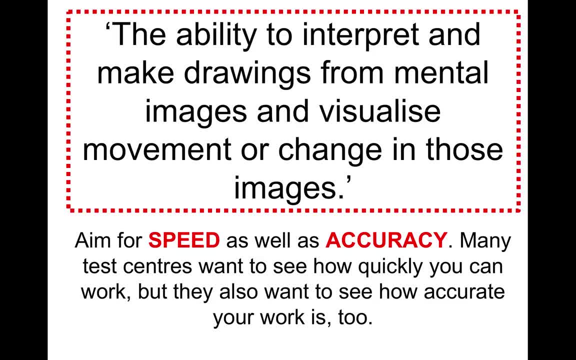 but also accuracy. So what you don't want to do is work through the exam and then start guessing if you're unsure, because many test centers can deduct marks for guessing or inaccurate results. So let's say there's 30 questions in your exam. 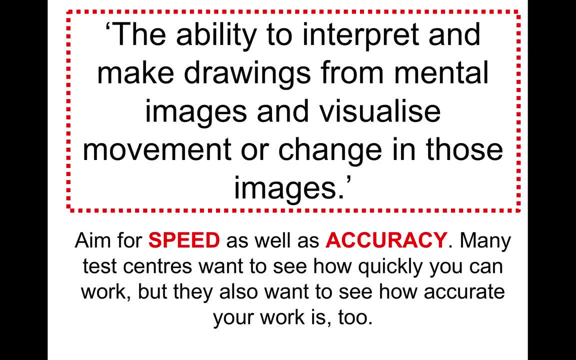 OK And you get 15 correct and you get 15 wrong, You could lose marks for those 15 incorrect ones. It's better off not finishing the exam but getting, say, the 13 that you do attempt correct. OK, That's far better. So you have to aim for speed, but don't be worried if you don't. 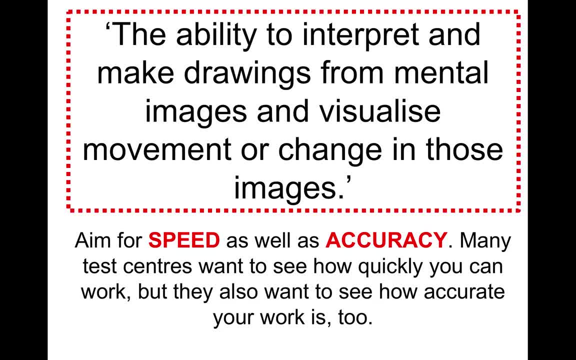 finish the test, unless specifically they say to you you have to finish this exam. Most of the spatial reasoning test questions in the exams that you'll undertake are very difficult to finish. OK, So it's designed to put you under pressure, So stay calm. Yes, you have to aim. 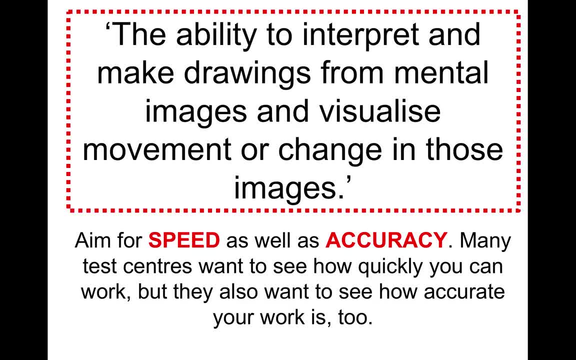 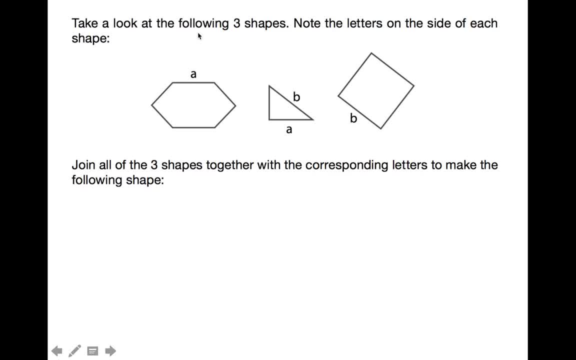 for speed, but accuracy is really important. Let me get into a few sample questions and answers and explain how to tackle them. So if we take a look at this sample question, take a look at these three shapes, OK- And take a note of the letters on the side of. 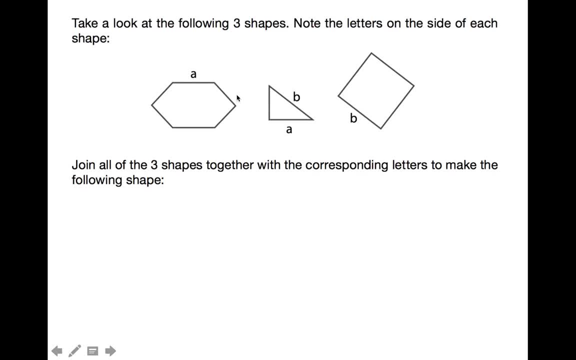 the shape. So you can see on A there, B there, A at the bottom and also B there on the side. Now your job is to match them up Together with the corresponding letters to make a shape. So if we take a look at the level there, 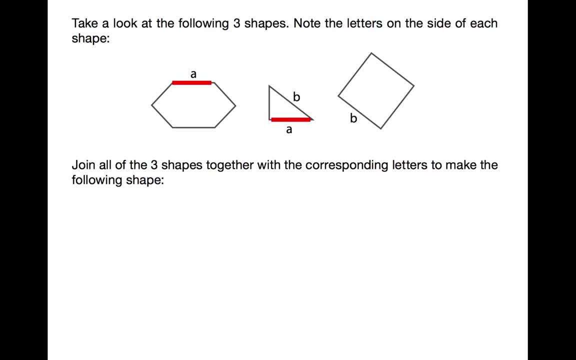 on point A: OK, And also the level there. on point A, We have to match those together exactly, And the same applies to point B on both of those shapes. So if we actually match them together, then that is the shape that we would get. More often than not, these kind of tests are multiple. 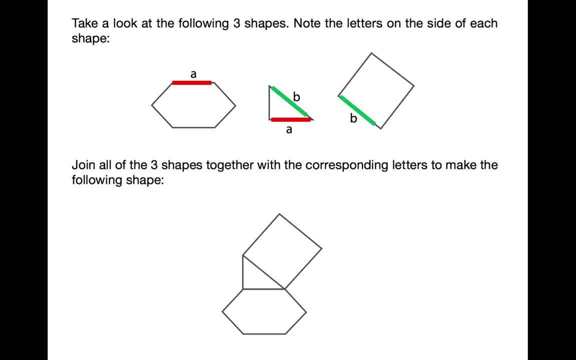 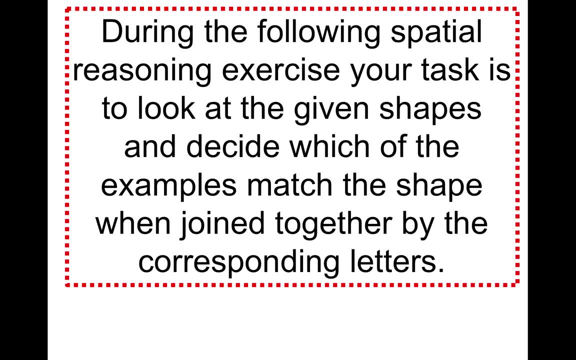 choice in nature. OK, You have to pick out which is the correct one. So I'm going to give you an exercise now, a spatial reasoning exercise, and it's your job to look at the given shapes and decide which of the examples match the shape when joined together by the corresponding 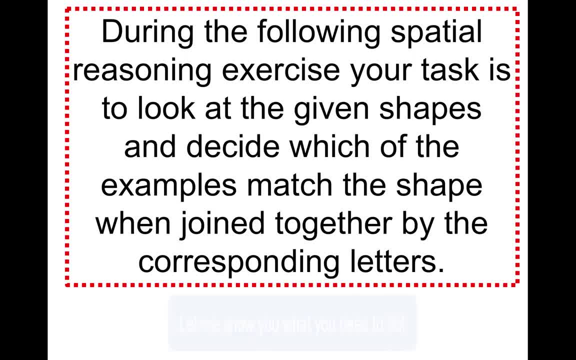 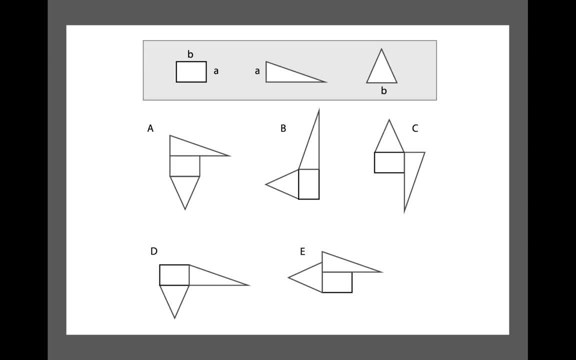 letters Very similar to what I've just shown you. So what I'm going to do is let me show you what you need to do. So this is the kind of question that you might be presented with. And again, you can see across the top. you've got the shapes, you've got a rectangle with. 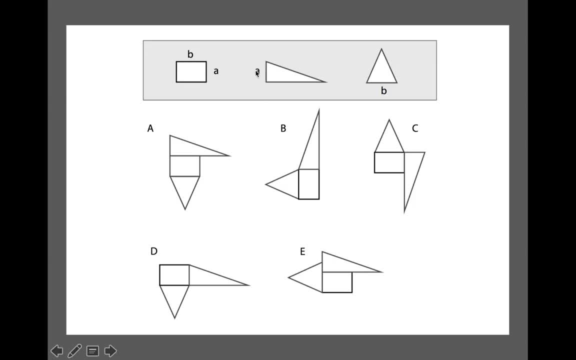 B and A next to it. You've then got a triangle. You've got a triangle with A on it and another triangle which has the letter B on it. You have to match all of these up exactly as they are and then decide which after the multiple. 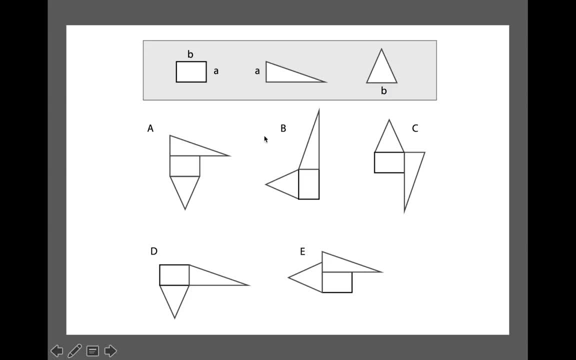 choice options A, B, C, D and E is the shape when they're all brought together. So if we take a look at point B there and point B there, if we match those together, you can see that's what the shape would look like. Now what we can do here automatically is we can dismiss. 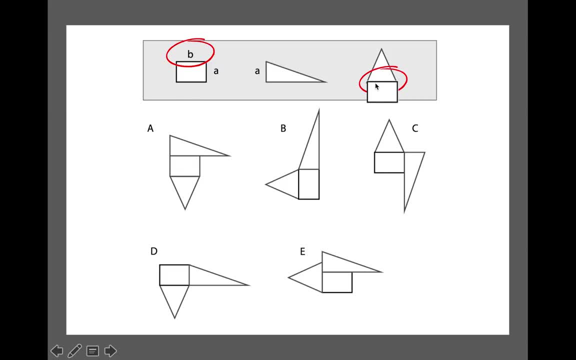 those, because all we have to do is rotate in our mind, either clockwise or anticlockwise, which way this would be. You can see that C has this shape as part of it, B also has that shape there as part of it, A does, and D too, but E doesn't. So we can automatically 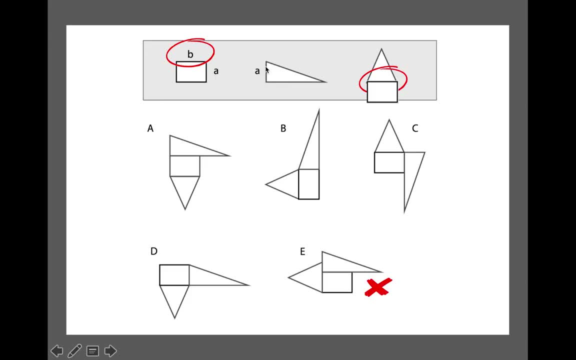 dismiss E. Okay, Now the next part is to put point A there at the top, next to that point, And that would give us that shape. Okay, That would be the shape Now we have. We have to do this visually and mentally in our minds. 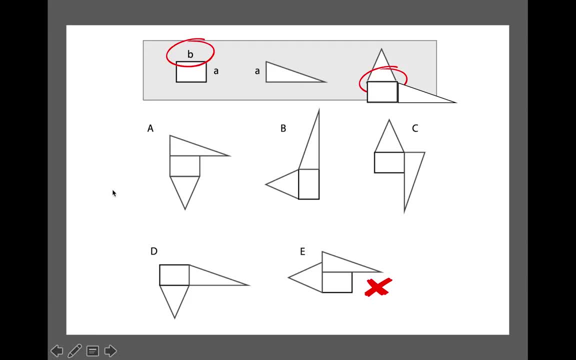 And then we have to work through A, B, C and D, Which is the correct answer. So we can automatically see that it's not A, It's certainly not D, It's not C, So the correct answer is B. Now you will note that D and B are very similar, and that will probably 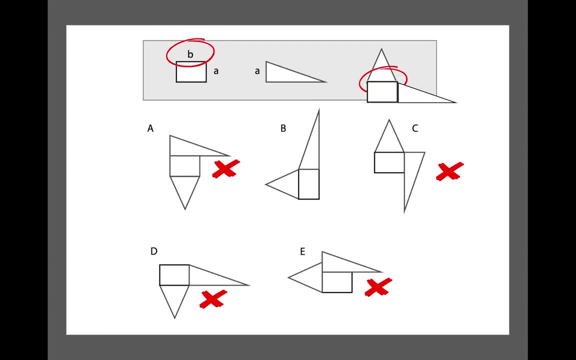 happen during the multi-choice options is that some of them will be quite similar. to try and catch you out, But the correct answer there is obviously B. Now what I want to do is give you a few of these yourself to have a go. 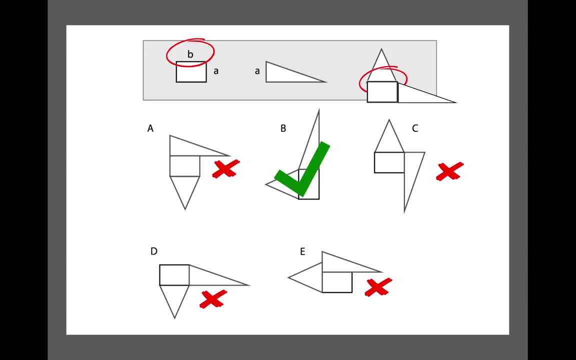 So watch them in real time, Each of the questions. you're going to get 20 seconds, okay, and you'll notice a blue circular timer, either in the bottom left hand of your screen or the bottom right, And when it comes round to the full circle, the 20 seconds have run out and I'll give. 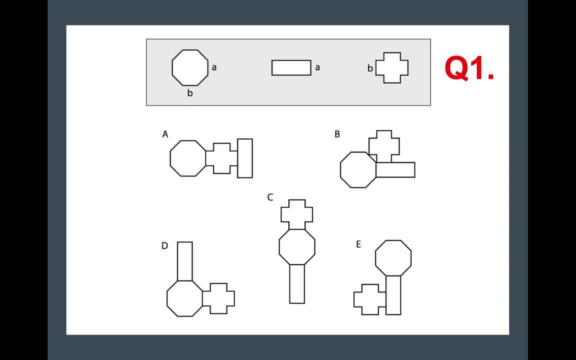 you the answer. So this is the first question, question number one and your idea- sorry, your aim is to put all of these shapes together with the corresponding letters and then decide out of A, B, C, D or E is the correct answer. 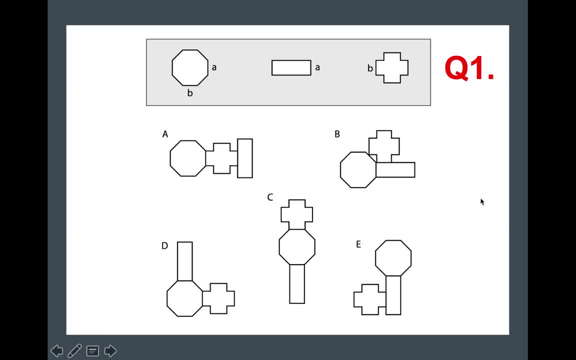 So I'm going to start the clock and you have 20 seconds to come up with the correct answer. Off you go And that's the 20 seconds up. So how did you get on? Were you able to dismiss some of the questions quickly, some of the shapes and the options? 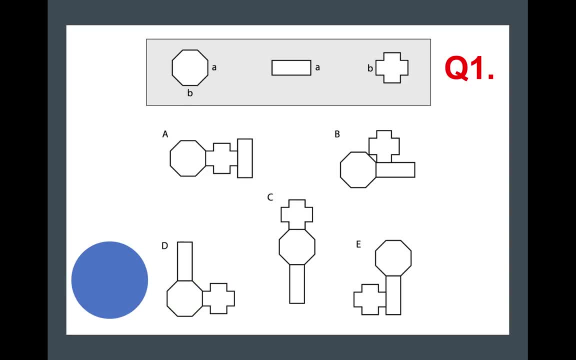 quickly. The correct answer is, of course, D. Okay, that is the correct answer, So hopefully you got that question right. Let's now move on to question number two in the series. Now again, I'll start the timer and you have to decide. you can see the different shapes. 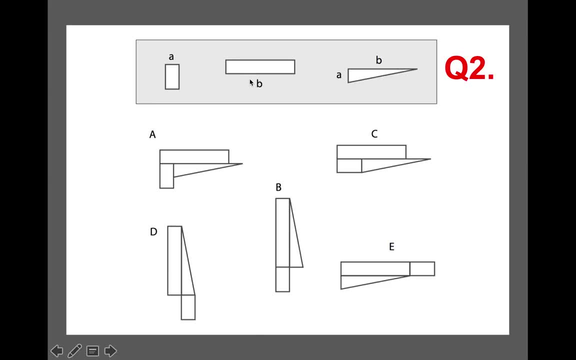 and the different options with the corresponding letters, Which is the correct shape out of multiple choice options A, B, C, D and E. So I'll start the timer and you've got 20 seconds to come up with the correct answer. So hopefully you've got the correct answer to the question. 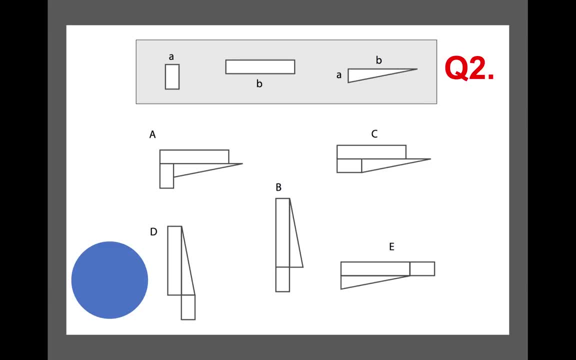 Excellent, Well done. So hopefully you've got the correct answer to the question. So if I was to put A there, I would have a long talk. I would have the long talk. So I'll just give you the answer. You can see from the bottom here that the A, B, C, D or D are very similar. 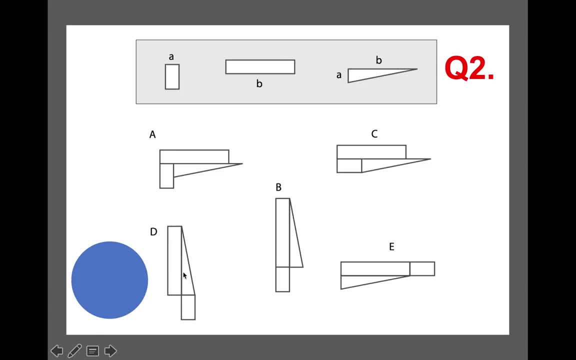 So the answer is B And you can see these are very similar. The only difference between these two is that small rectangle is perched on the bottom of the triangle and there it's perched on the longer rectangle. Okay, so it's very easy to get one of those incorrect, and the actual correct answer is: 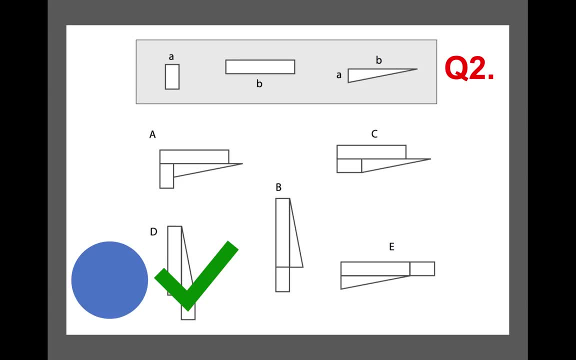 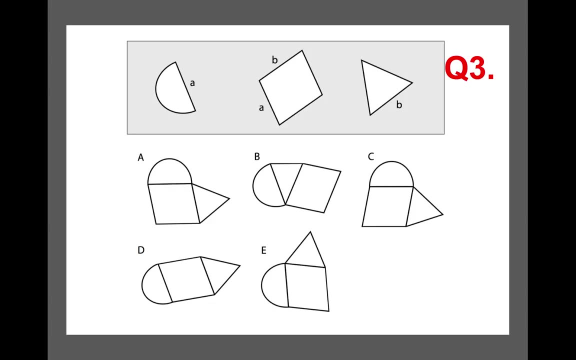 of course D. Okay, so that's the correct answer. So let's move on to another one. You see, these shapes were starting to get a little bit harder, a little bit tougher. Now the timer will appear in the bottom right hand corner of the screen, this time. 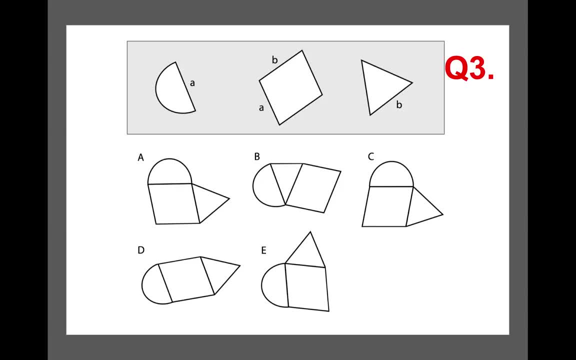 So decide which shape out of A, B, C, D and E. The correct answer is: when you join all of these corresponding letters together to form one shape, Off you go. So I'm sure you will have found that one a little bit tougher than the previous ones. 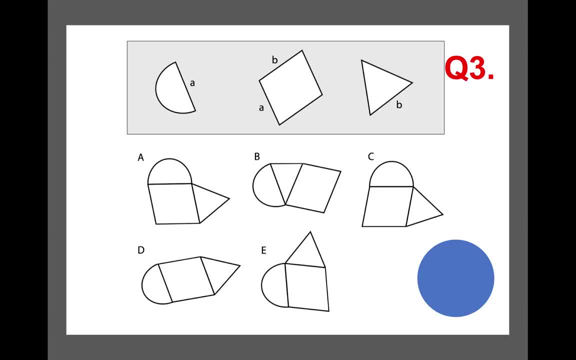 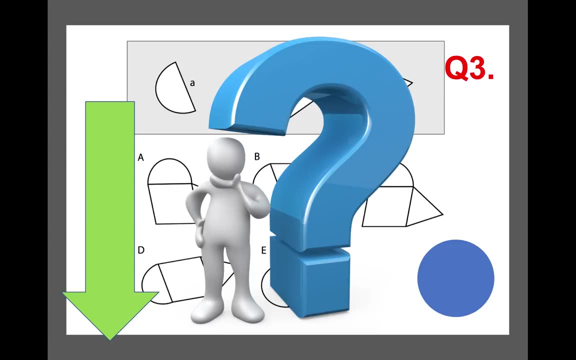 because the variations in the shapes they look different. It's not what we're used to, And you also have to rotate them around visually in your mind. So what I want you to do is to tell me which is the correct answer. Okay, and I'd like you to do that by putting your answer in the comments section below. 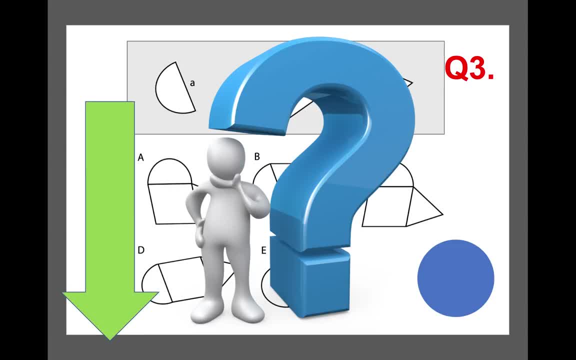 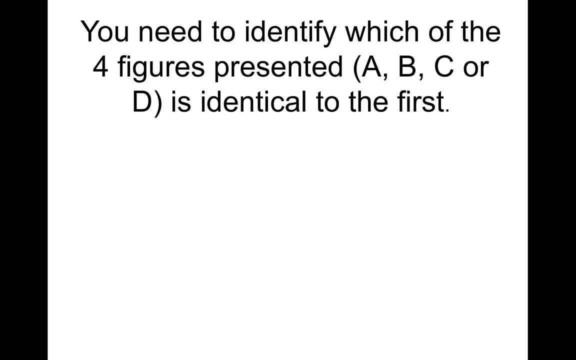 the video. Okay, so put your answer in the comments section below the video now, and then I'll mark it for you and let you know if you are correct. Okay, so those are like combining different shapes. In this second type of spatial reasoning test, you need to identify which of the four figures. 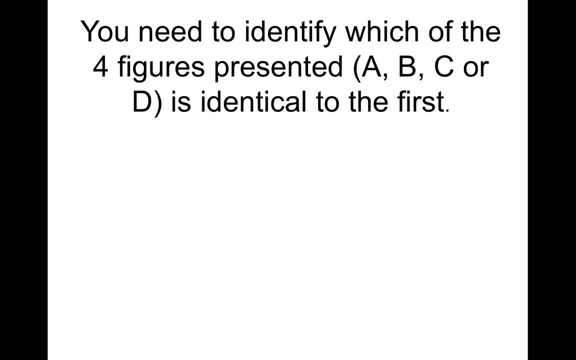 presented again multiple choice. A, B, C or D is identical to the first shape. So this is the first shape and you'll notice that there are a number of different shapes around a central theme. So if I show you the four different options, we need to identify which of the four figures 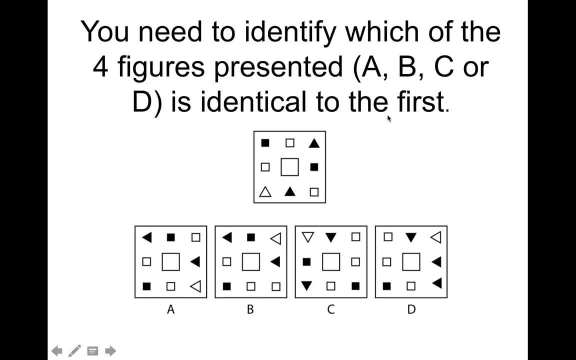 presented- A, B, C or D- is identical to the first one. Now, when you look at these on face value, it can be quite confusing, and when you're doing lots and lots of these tests, your mind can become confused and you just start to. 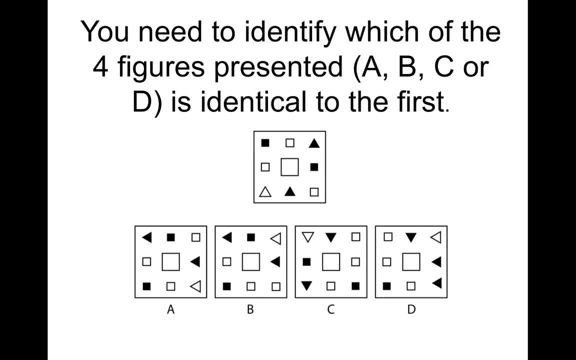 see a mass of shapes and dots and figures and you start to panic. What you should do in this kind of question is to just focus on one row. So if I just focus on that row there and not worry about the others, and then come down, 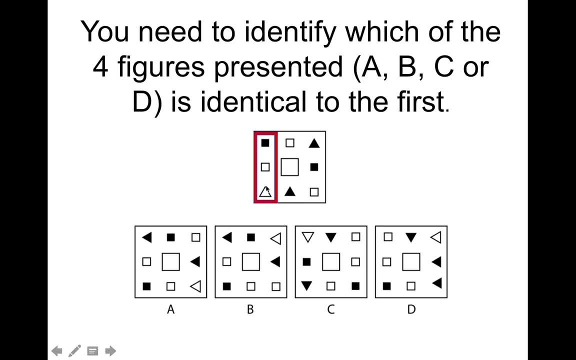 to A, B, C and D and try and find that one sequence. I just need to find that one sequence where we have a blank or a white triangle, a blank or a white square, And then I'm going to try and find that one sequence where we have a blank or a white. 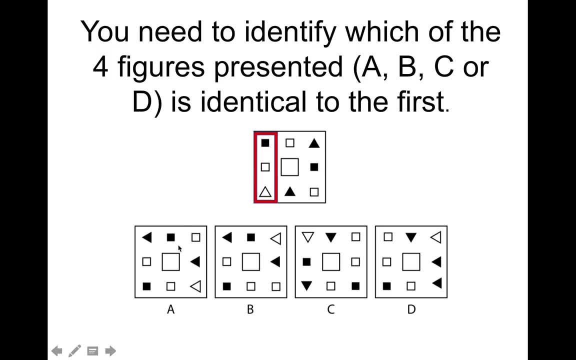 triangle, a blank or a white square And then also a black square. So if I look along these shapes- and it can be from the bottom going up or at the top or the side, and the only one where I can actually see this on all of these shapes is 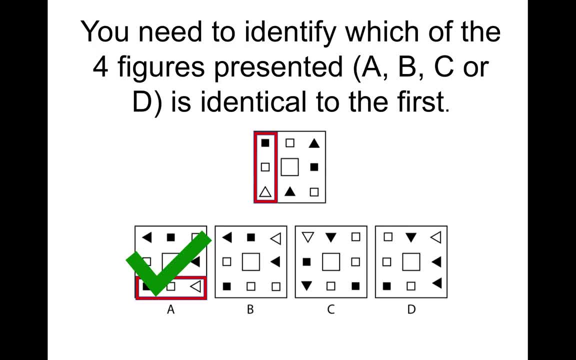 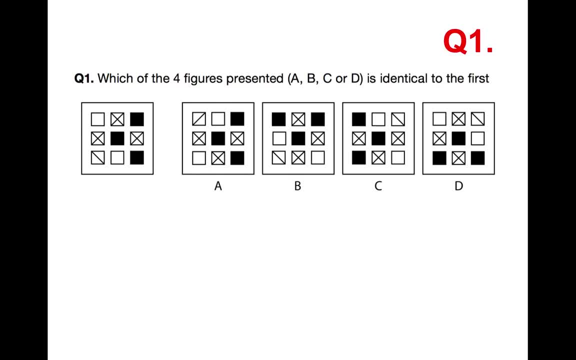 in A and therefore A is the correct answer. Okay, So A is the correct answer to that. So what I'm going to do now- same again- is I'm going to give you a series of questions. I'll set the timer. 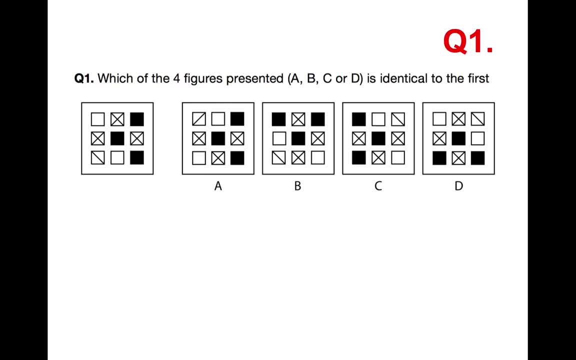 You've got 20 seconds to come up with the response, and then we'll take a look at the correct answer. So you've got 20 seconds to find out which of the four figures presented is identical to the first one on the left. 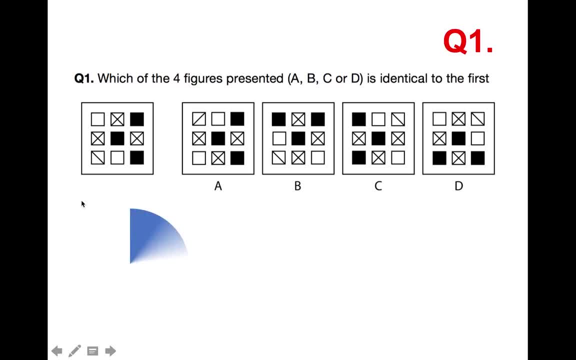 Off you go. Okay, well done. So you can see that there's lots of different shapes there. The correct answer is, in fact, C. Okay, now what you'd have to do is move this around mentally in your mind and keep everything in the same place. but you can see that place. 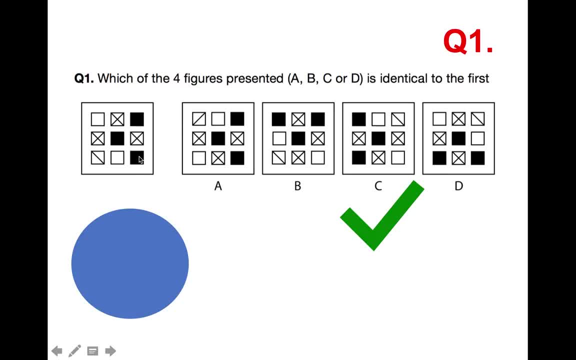 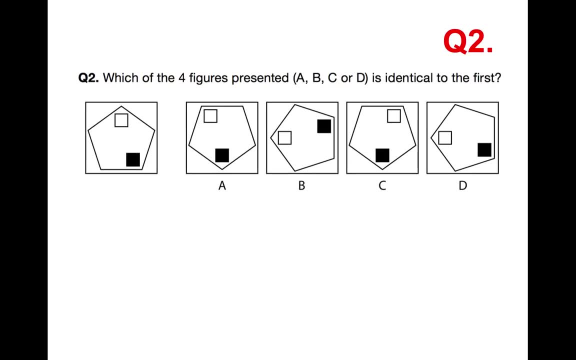 when it is rotated through 180 degrees, clockwise or anti-clockwise. we come up with that shape there. So let's take a look at question number two. You've got some different shapes now, slightly easier, I would suggest, but which of the 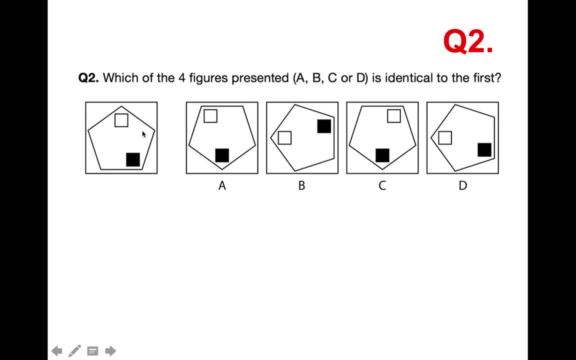 four figures presented: A, B, C or D is identical to the first on the left-hand side. you've now got 20 seconds Off, you go? Okay, well done, and I'm sure most of you got that correct. The correct answer is B. Now what I want to mention at this stage is there may be a. 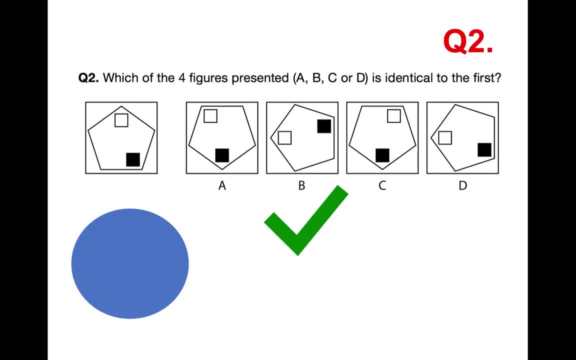 variation In the kind of question where it might give you a fifth option which is none of these- Okay, so you might get figure A, figure B, figure C, figure D, and then E might be none of these. Okay, so you might get an option where none of them are correct. 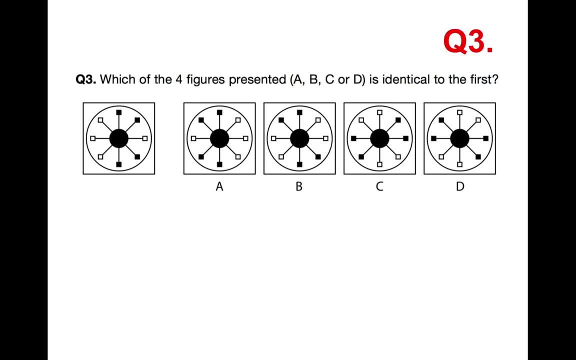 So let's now move on to question three in this type of spatial reasoning test question. So which of the four figures presented- A, B, C or D- is identical to the first? Don't forget, you've got a 20-second timer. 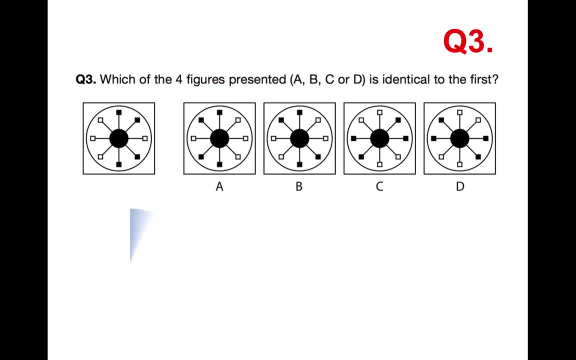 Okay, And then we'll go through the answer Off we go. Okay, well done. So how did you get on with that question? Slightly harder or much harder, Because you've got to look at all the different variations. Okay, well done. 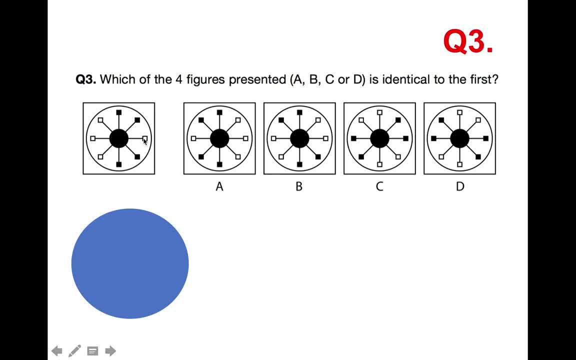 You've got to look at all the different variations With the black squares and the white squares. there's obviously four of them in there, four there, but what's the difference between the two there? there's three there, so you're trying to find a sequence with three so you can automatically dismiss B. You can even. 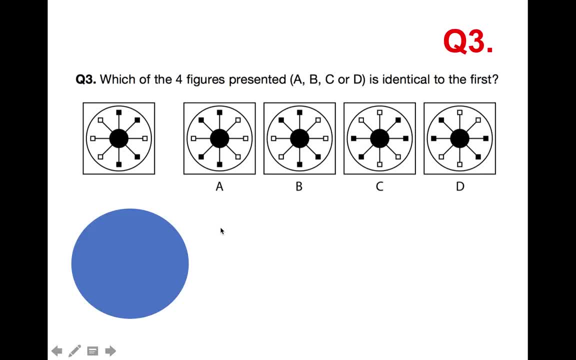 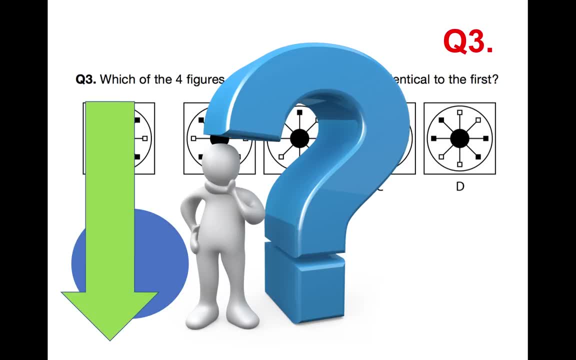 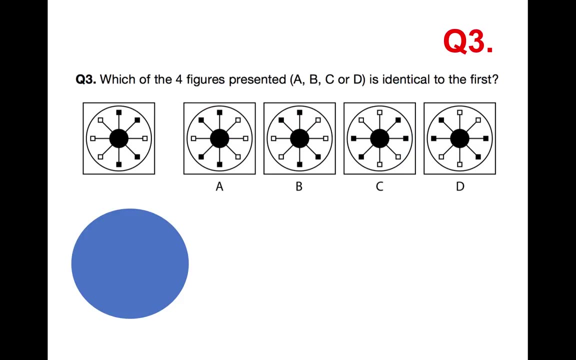 dismiss that one. So let me know which question- sorry, which answer to question three- is the correct one, And please once again put your answers in the comments section below the video. Let me know. Let me know the correct one of those four figures presented- A, B, C or D. that's identical. 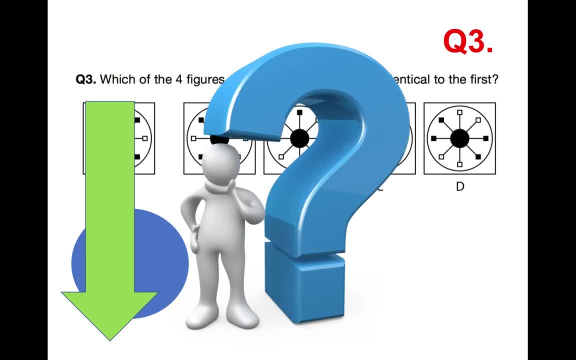 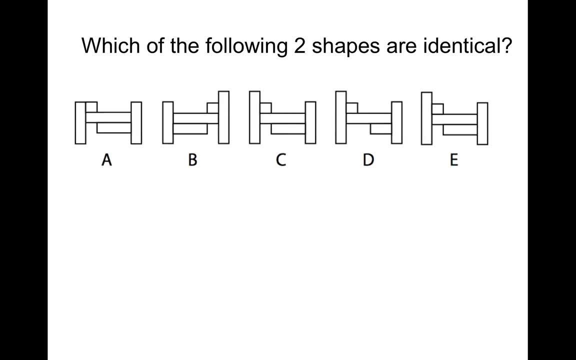 to the first on the left. Okay, Now let's move on to the next part, the next kind of spatial reasoning test question: Which of the following two shapes are identical? So you're presented with a series of shapes- A, B, C, D or E- and you have to decide which. 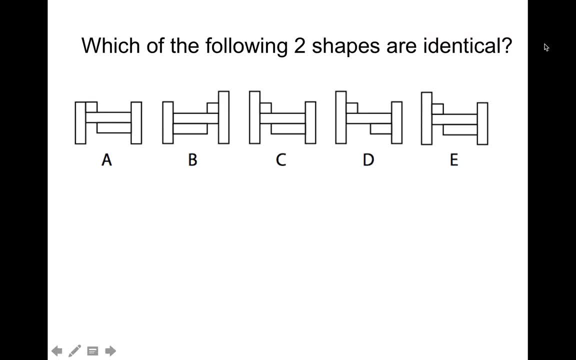 of the two are identical, so you have to do a little bit of working through them to see which is the correct one, And the answer here is C and E. C and E are identical. So again, we'll go through some sample questions. 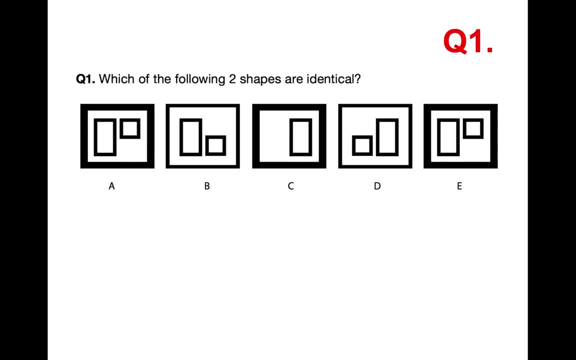 You can work them out with the 20 second timer. So which of the following two shapes are identical? You've got 20 seconds starting from now, So that question was quite easy to start off with to get you going, and the correct. 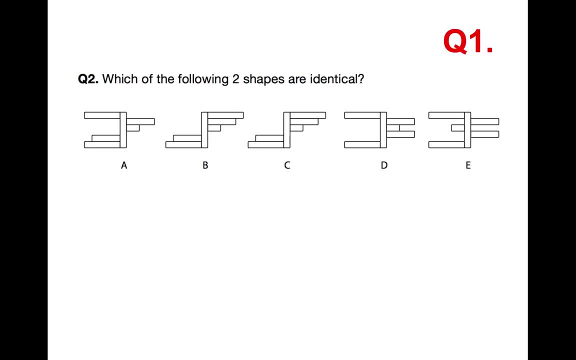 answer is A and E. Now let's move on to question number two. Which of the following two shapes are identical? You've got 20 seconds starting from now, Okay? So of course you would have seen that the correct answer is B and C. Now the third one.